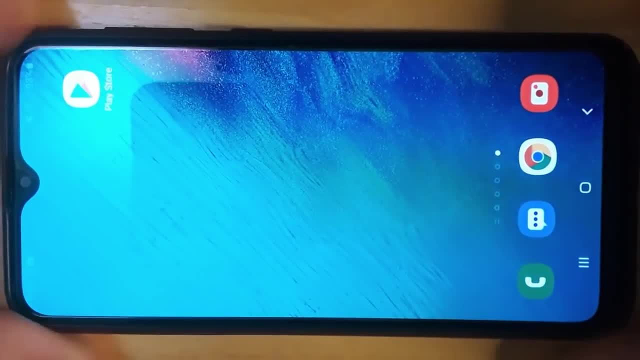 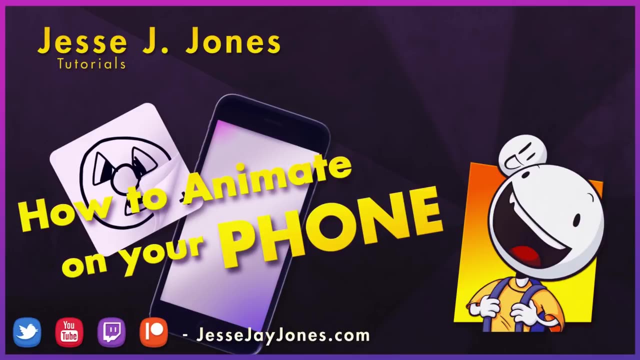 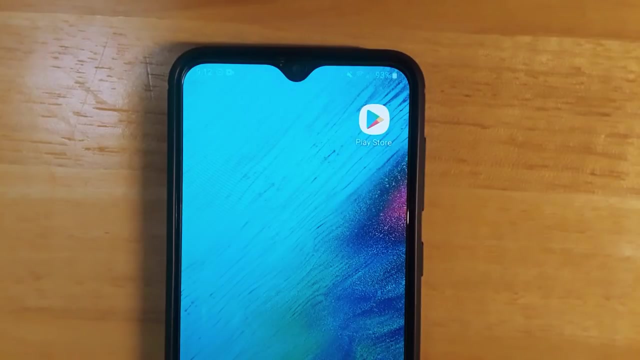 In today's tutorial, we will learn how to animate using nothing but our phones, And the example I'll be using is an Android phone, but this will work for iPhones as well, So the app I'm going to be using for animating on our phones is called Flipaclip. 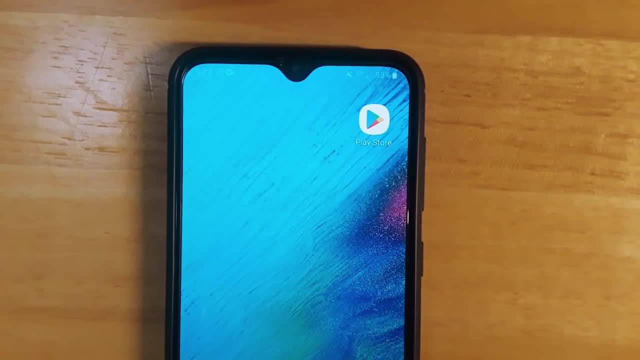 There's also other apps that I would recommend, like Rough Animator, which is about $5 and is also a very good app and also Procreate, But in this tutorial, Flipaclip is free and pretty much accessible to everyone, so that's the one we're going to use. 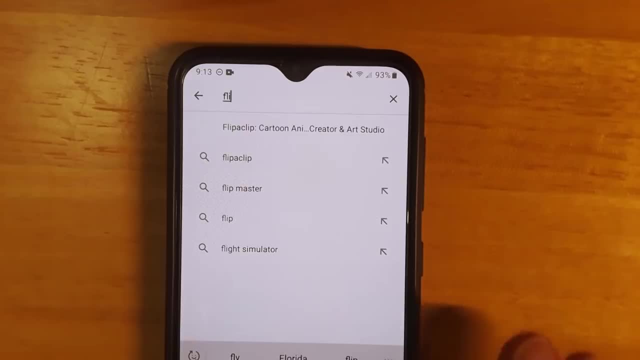 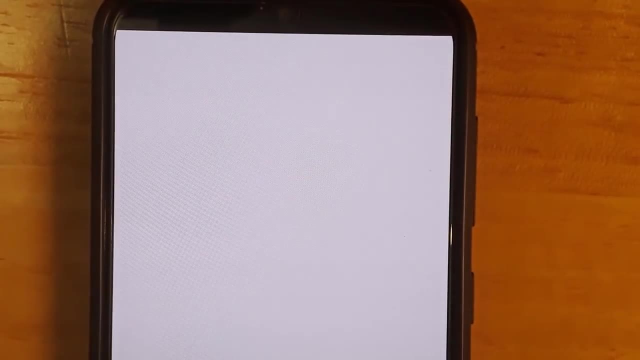 So we're going to open up our App Store and we're going to type in Flipaclip to download it, Then click the Install button. So now that you've got Flipaclip downloaded, let's open it, And I'll just turn my screen horizontal so we can see what we're working on. 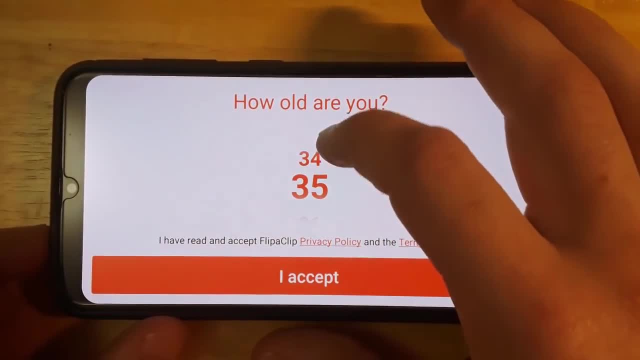 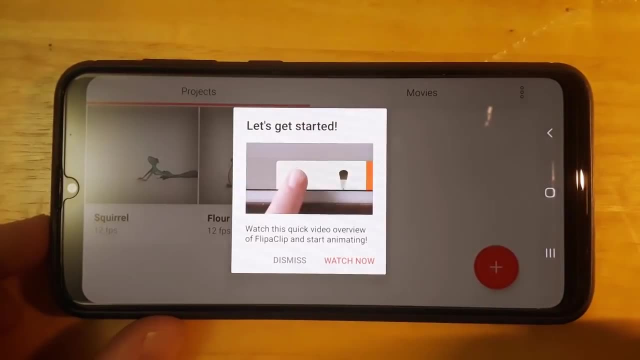 It'll ask some questions when you're first installing. I don't want to give away how old I am- 34.. But um, And then, when it first starts up, there's a little tutorial. I recommend checking out its default tutorial, just so you get familiar with how to use all the tools. 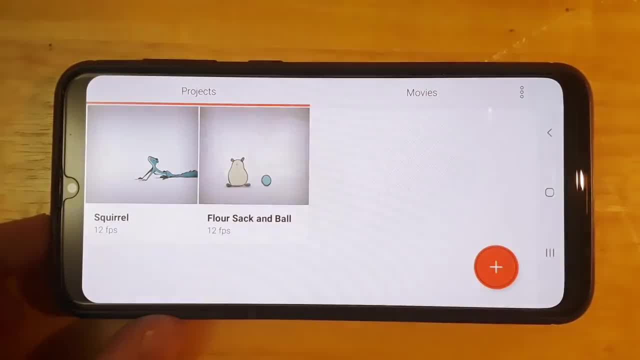 But we'll also go over the tools in this video, So I'm going to click Dismiss for now. So to start a new project, we're going to click on the plus button to create a new project. Give a name to your project. 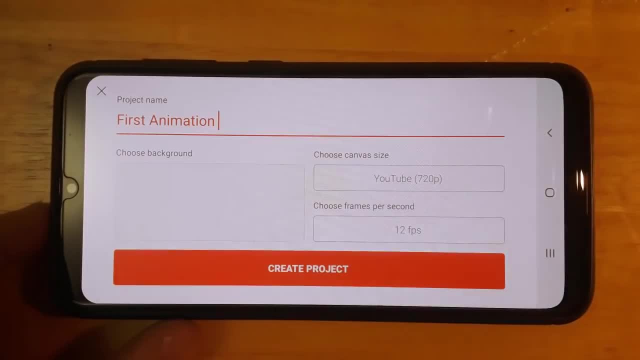 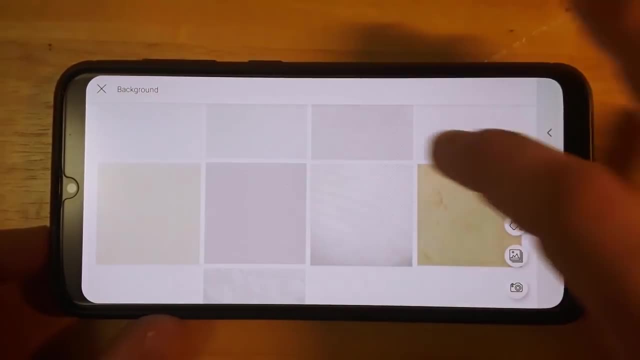 We'll call this one. First Animation, Click Done, And then we can choose a background for our animation. So it comes pre-installed with all these backgrounds already loaded onto it, Or you can use the paint bucket to select a color. use the image gallery. 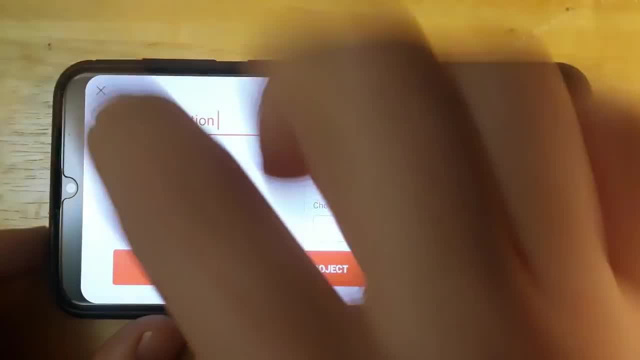 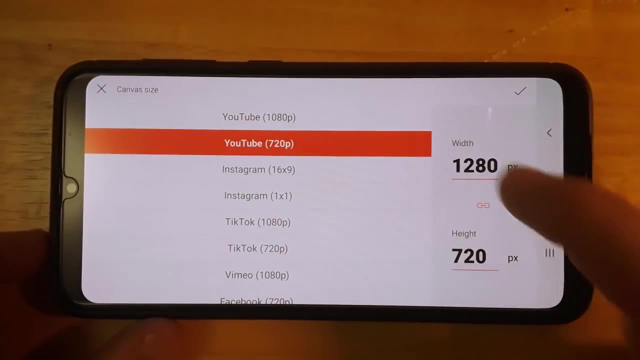 or you can take a photo with your camera, But we'll just leave it blank for now. And then for the canvas size, you can select all these different default options. I'm going to select YouTube 1080p because that'll give us the highest resolution for our project. 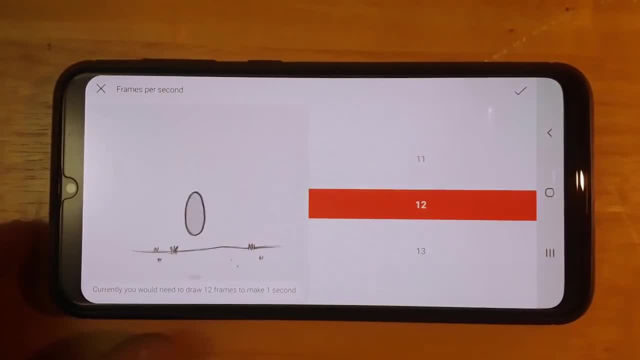 Then click the check mark to say OK. And for frames per second. you can think of this as how slow or how fast your animation is. So for this project we're going to do 12 frames per second. I recommend starting this way because it'll give you a nice smooth animation. 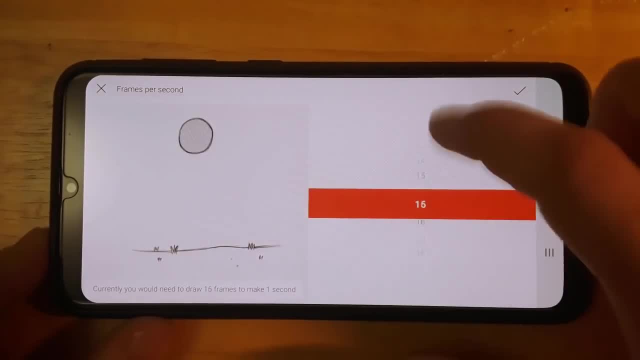 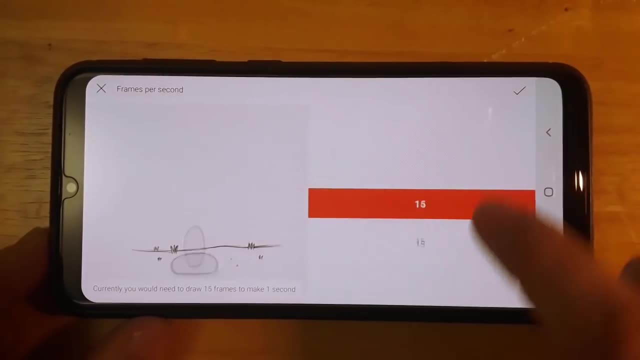 but you also won't have to draw as many frames. If you're OK with drawing a lot of frames. 24 frames per second is pretty standard as well, And it'll give you a nice smooth animation. So we'll set our project to 12 frames per second. 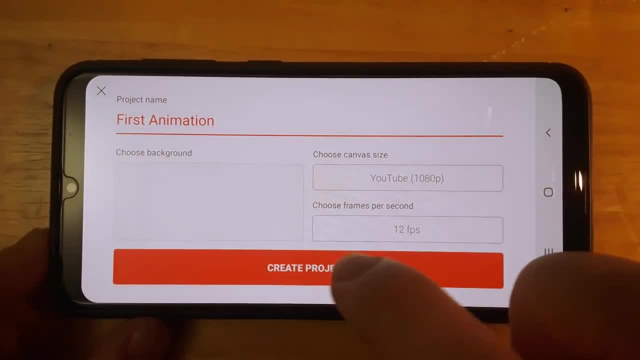 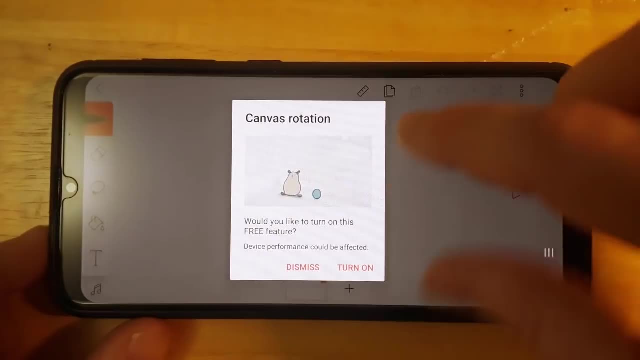 Press the check mark And we're all ready to go. So select Create Project And we have our project created. So for some phones, you'll be able to rotate your canvas using your two fingers and rotating. Some phones will not be able to support this. 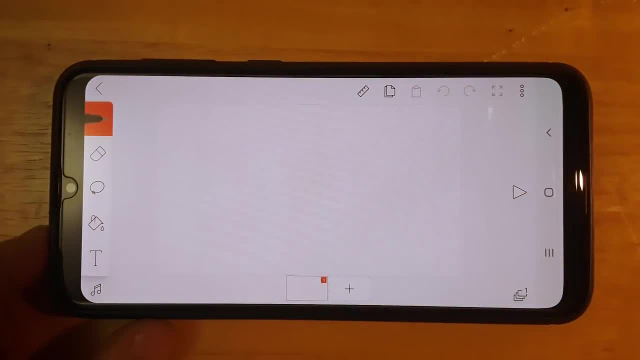 but we'll turn it on for this example, just so you can see what that looks like. And when you first open up Flipaclip, all your tools are on the left side, Your animation timeline is on the bottom, Your layers is on the bottom right. 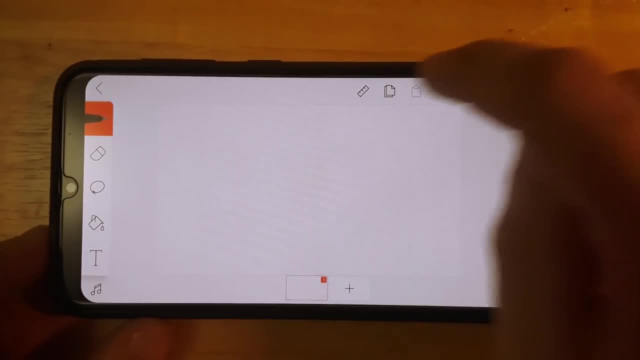 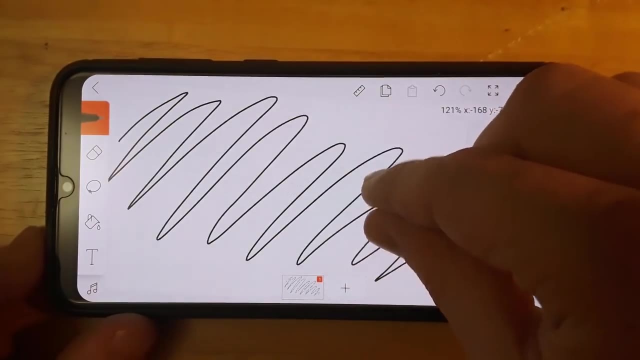 And your play button for your animation is on the right. Then you have your tools for your canvas on the top right. To move around your canvas in Flipaclip you can use two fingers to zoom in and out And you can also rotate it, if you enabled that option before. 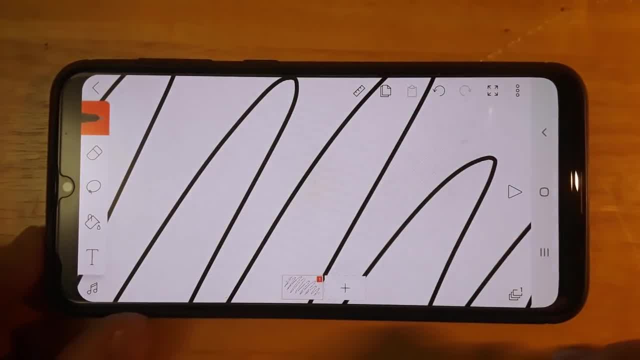 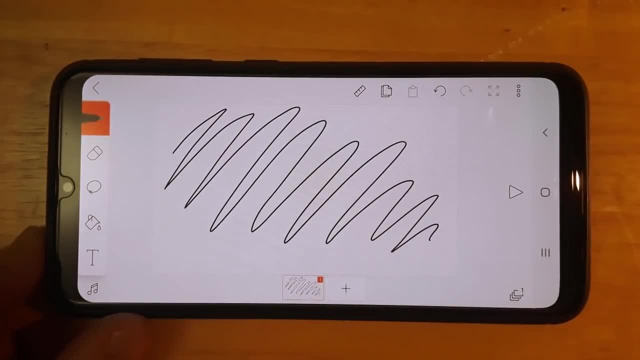 So zooming in can be really useful for drawing, like fine details, for example, And to zoom back out, you can select this four arrows on the top right here And that'll reset your view back to 100%. So the pen is selected by default when you first start out. 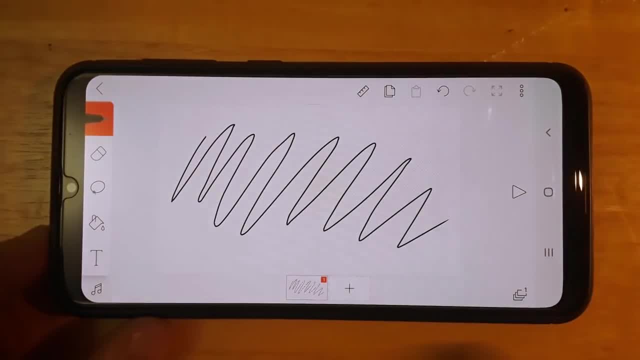 And if you select with your finger and just start drawing, it'll start drawing for you. If you want to undo, just click the backwards button here And to redo, select the forward button If you select any of the tools after it's been clicked on already. 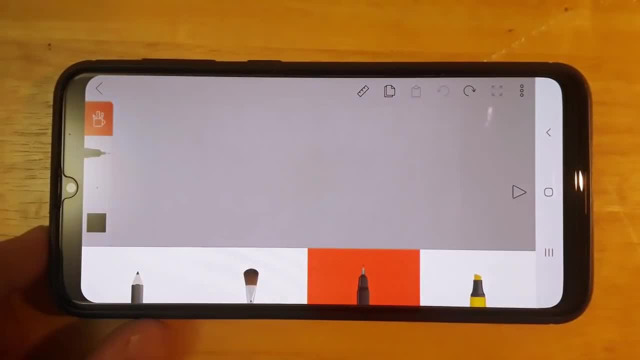 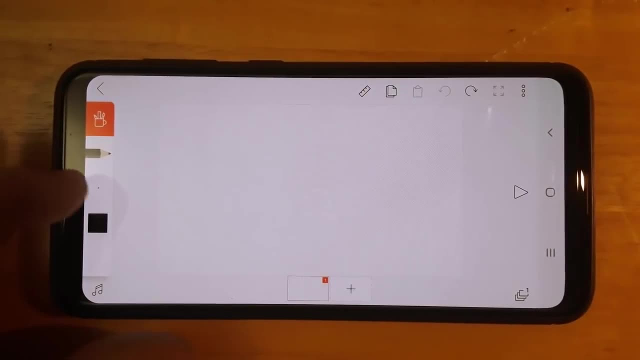 you'll get your options for your tools. So this top option, if we click it, we can select Pencil, Paintbrush or Highlight, And then the next option is the size of your brush. So if you press and hold you can see a little size option. 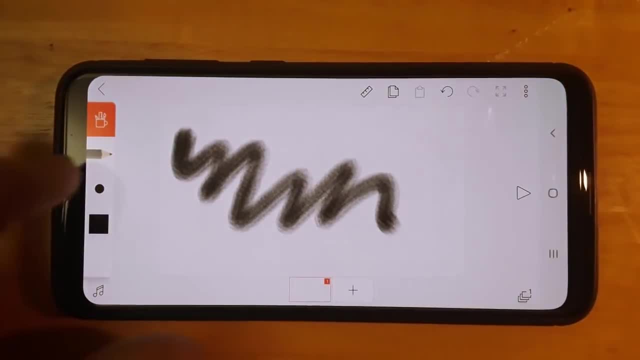 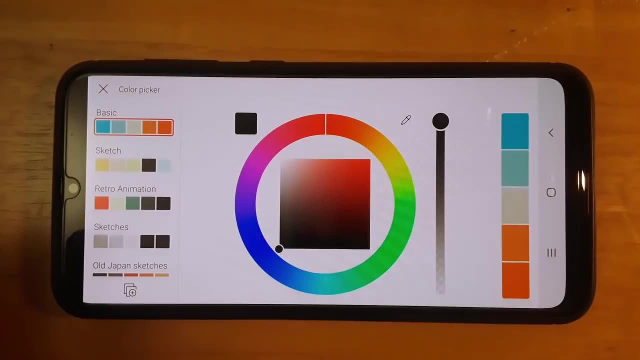 And then if you drag up, you can get a bigger brush. And if you select that circle and drag down, you can get a smaller brush, And then the square below that is how you select your color. So you'll see that it has all these default color palettes next to it. 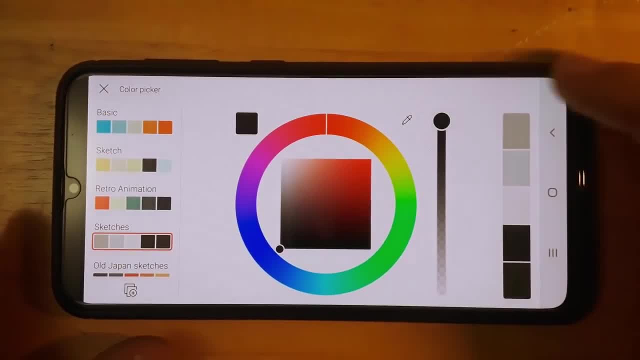 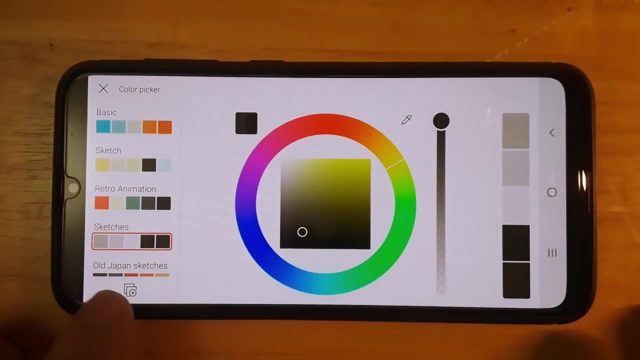 I like selecting the Sketches palette personally, And then you'll see these colors appear on the right, So you can select different colors on your palettes. Or you can create your own palette by clicking this Add Palette Button at the bottom of it. 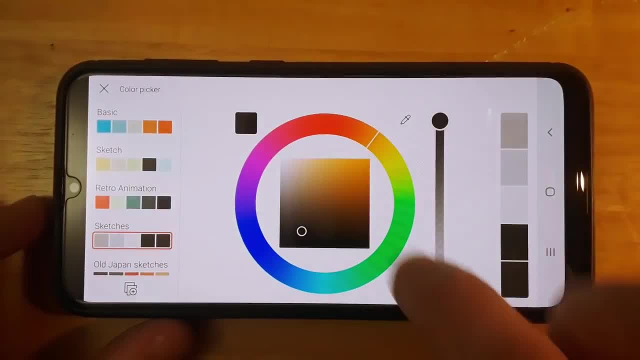 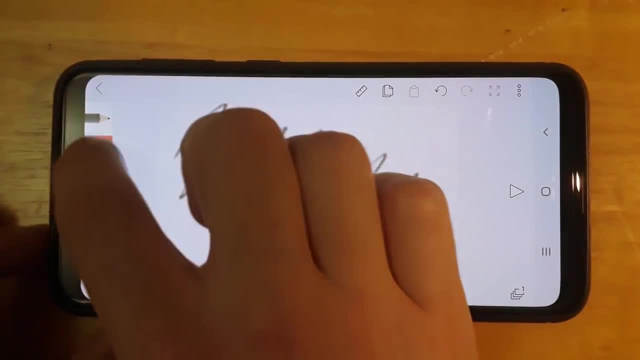 Or you can select what color you want on the outside ring and then selecting how dark or how light it is in the middle. My next tool is my Eraser, So I can select that and then select it again for the options, And again you have the size as your first option. 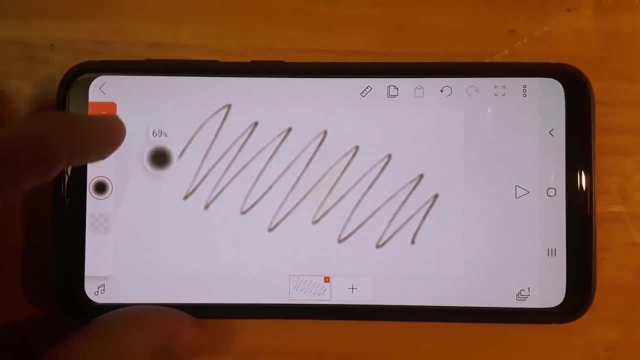 And then you have the hardness of Eraser as the next option. So it'll have either a really soft outline, so you can get really soft edges, Or, if you drag it all the way to the bottom, 50% of your lines are really soft. 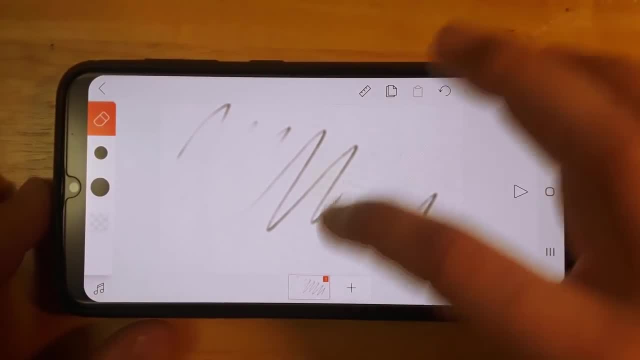 Also, if you draw it through the middle of the image, it'll give你就ix these contrast colors. Or you can create your own palette by clicking this Add Palette button at the bottom of it. you'll have really hard edges for really solid erasing. And then the next option. 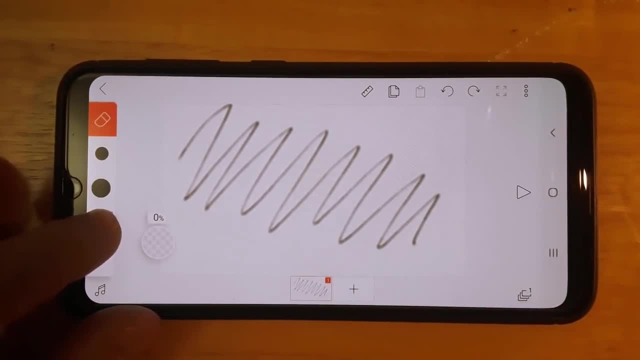 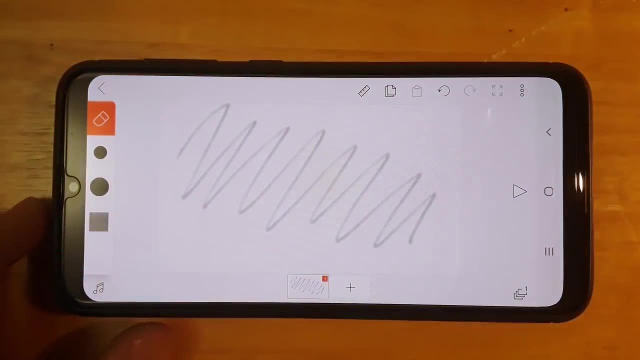 is the transparency amount. So if I didn't want to erase it completely, I could set this to say 50% and then erase it, and it'll only erase our drawing 50% of the way. There's also the paint bucket fill tool. so if I create a shape and 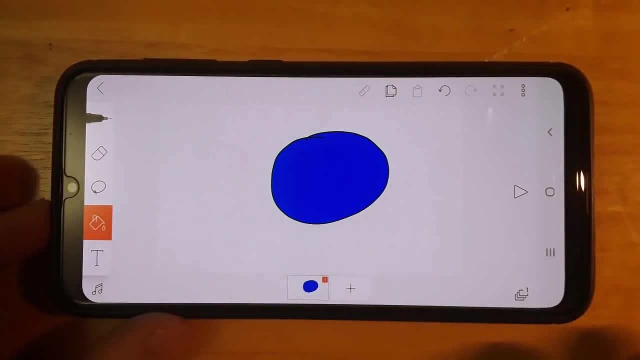 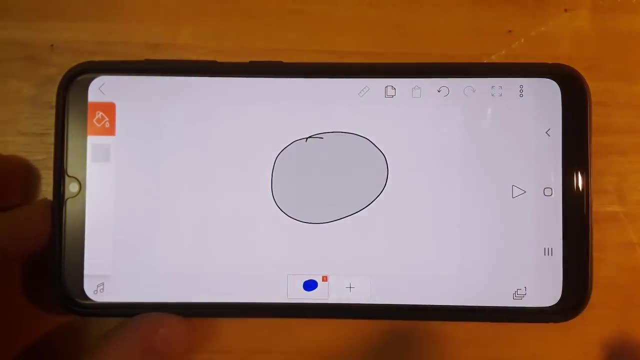 then use my paint bucket tool and press in the middle. it'll fill it in And again you can click on it again and then press the color button to select what color you'd like it to fill in with. The next tool I want to go over is the lasso tool. 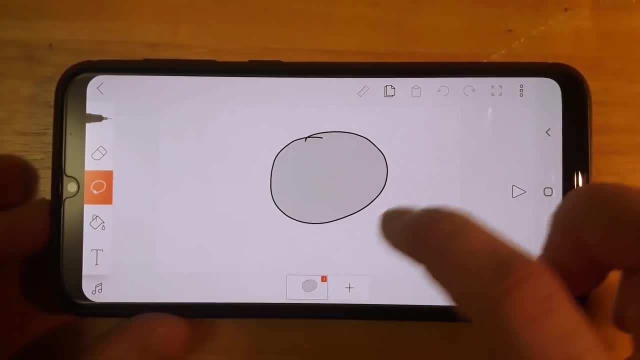 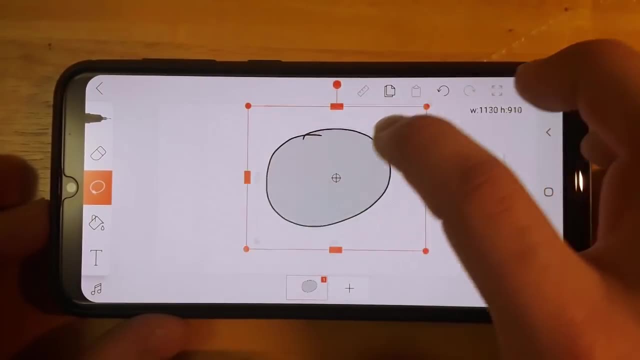 So the lasso tool is very useful. So what you can use it for is selecting a part of your drawing and then you'll see this transformation box around it So we can select our corners to scale our drawing, or we can select the sides to scale it. 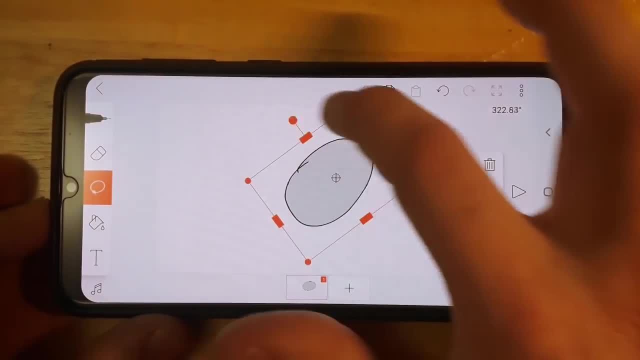 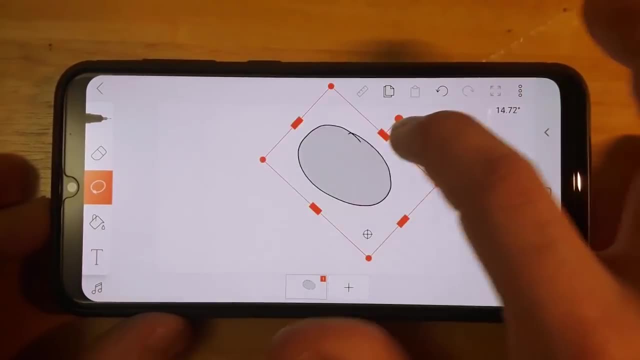 only on one side, or we can select this circle to rotate our drawing, And we can also move this anchor point in the middle here so that it rotates along a certain point of the drawing. So this is good for, say, moving arms around or moving the head around. 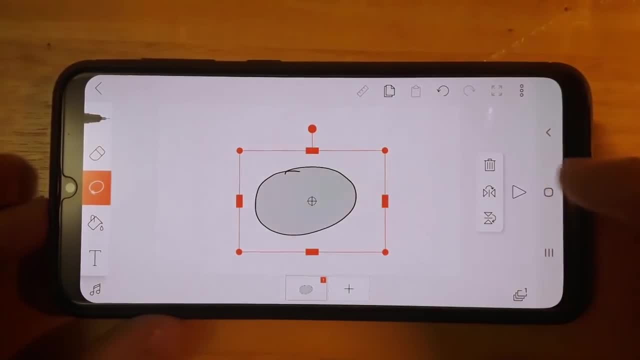 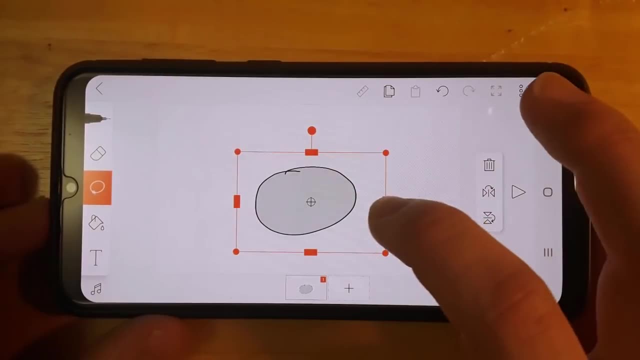 On the point where the pivot would be, which would be the neck, and you can also select: flip horizontal on the side here, or flip vertical, or delete it entirely with the trash can, When you're done transforming your drawing, just select off of it and the lasso tool will disappear. So the next thing I want to go: 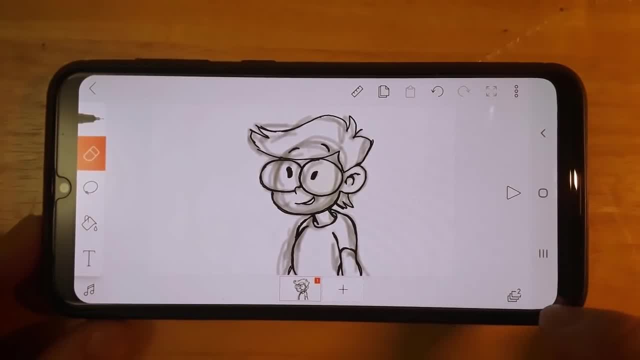 over is layers for your animation. So your layers panel is on the bottom right here, right where this stack of paper is, and that's kind of what you can think of layers as is stacks of paper. So if I select it, my sketch layer is on the. 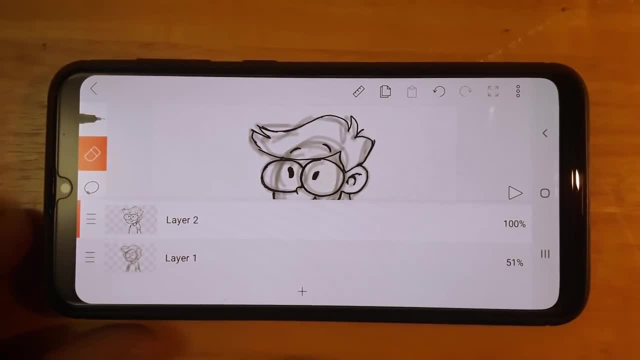 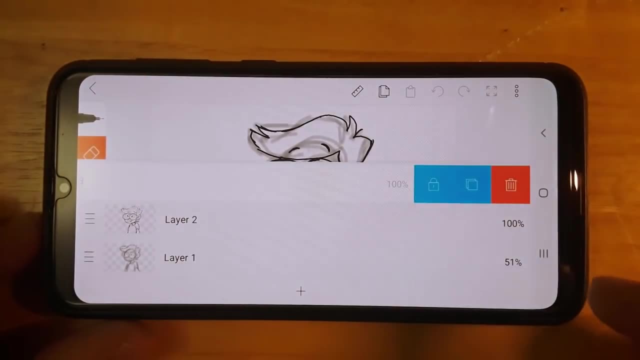 bottom here and then my ink layer is on the top. If I want to add a layer, I can just click this plus button on the bottom here and it'll add a layer. To delete a layer, I can swipe to the left and I'll get options to either lock the 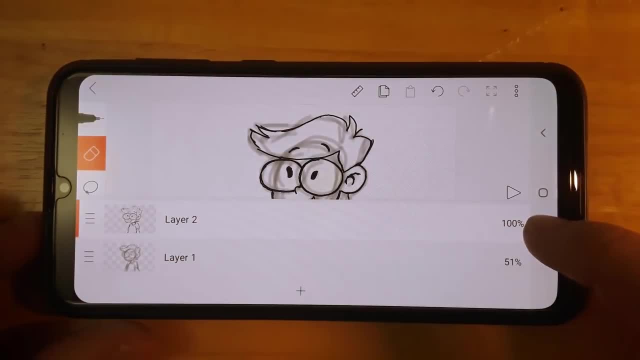 layer, copy the layer or delete the layer. If I want to change the opacity for a layer, like I did with my sketch layer here, I can press and hold and I'll get the same opacity slider. So I can drag up to make it more opaque or drag it down. 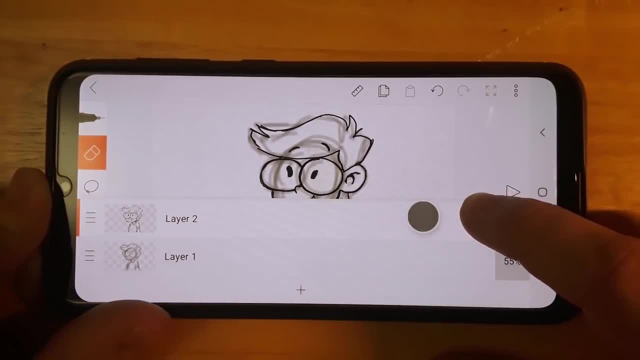 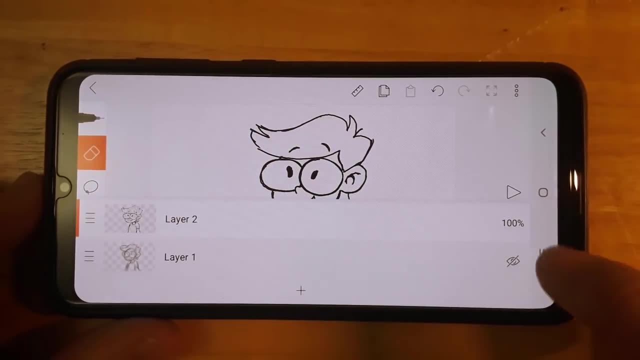 to make it more transparent. If I want to make it invisible, I can tap it instead of holding it, and you'll see a little eyeball with a cross through it showing that it's invisible, but it's still there. And to rename a layer, I can tap on the name and rename it. It's. 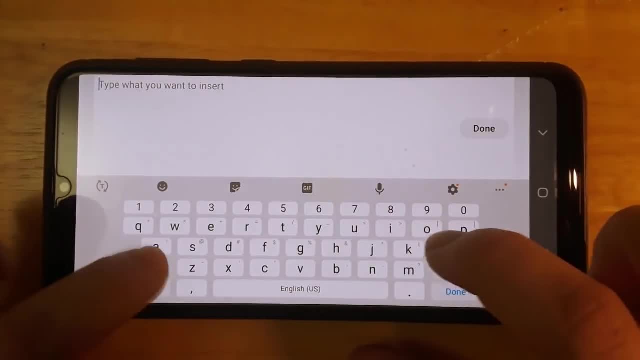 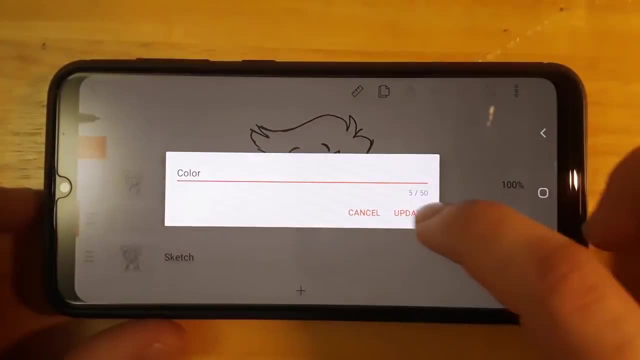 important to name your layers just so you have everything nice and organized- Always a good habit to get into. So for a quick example of how layers work, I can add a layer, call it color. so if I color in this layer, you can see the color is. 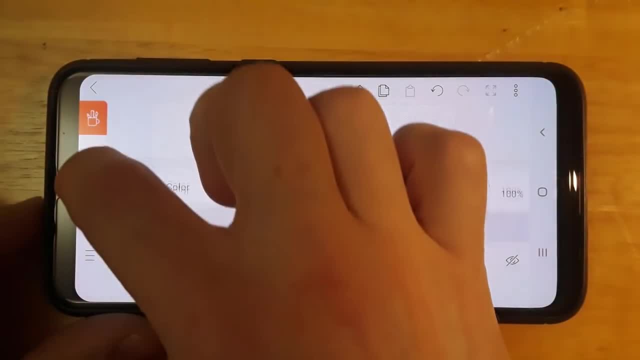 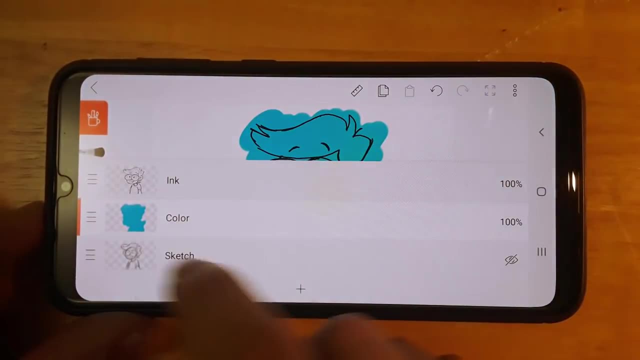 appearing behind the ink layer. But if I take that layer and drag it on top, you'll see my color is now in front of my ink layer. So this is typically how I like to arrange my layers. I like to have the sketch on the bottom at about 50%, my color layer in the middle and then my ink layer on. 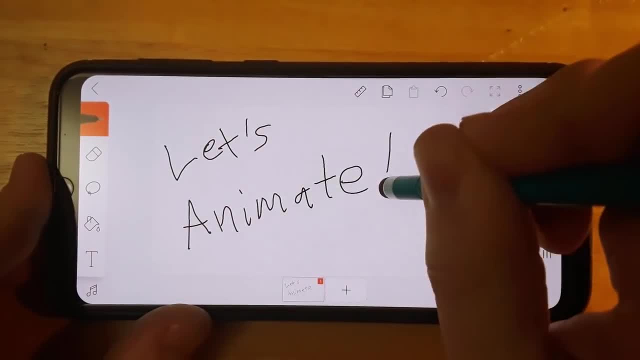 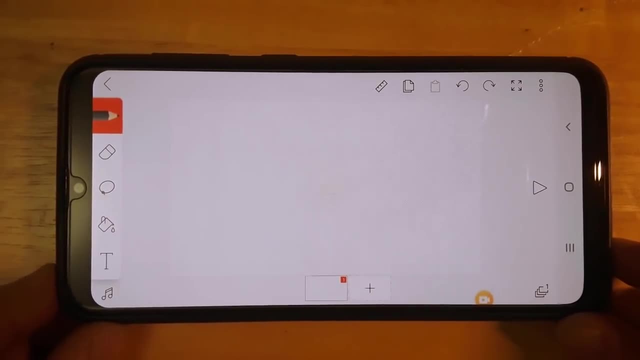 top. So now that we know how to draw and flip a clip, let's animate something. So the example we're going to use when we animate is a bouncing ball. It's a really great exercise when you're first learning to animate and it's kind of a. 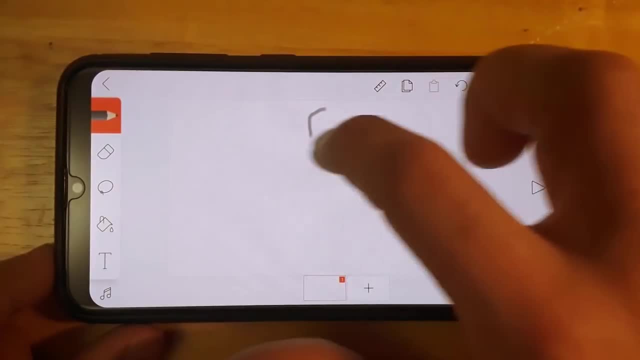 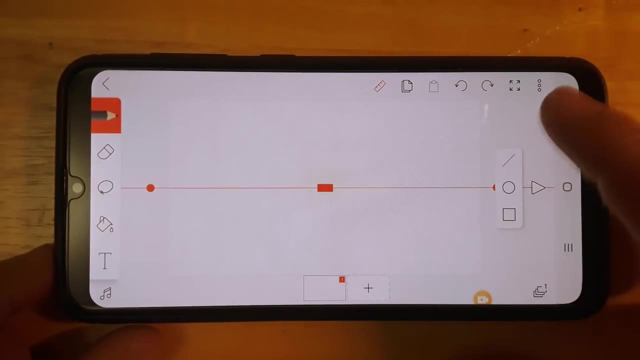 cool thing to show off once you're done. So, to start off, draw a small ball at the top of your canvas. Or if you're having trouble drawing a ball, you can use this ruler tool at the top here. and these are the shapes that you can draw with the ruler. So we'll select circle. bring in these sides to. 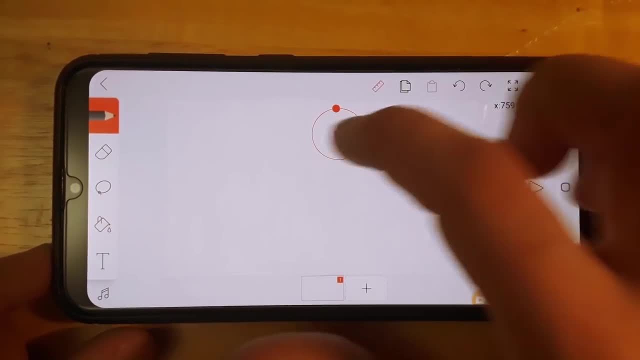 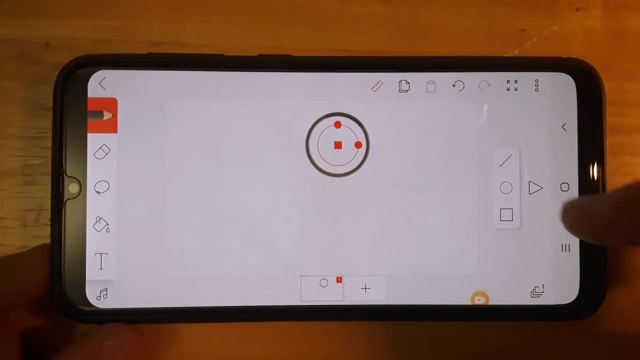 make the circle smaller and then drag it in place using the square in the middle, And then, whatever tool you have selected in your drawing tools, you can trace around the circle like so and you'll get a perfect circle. Then just click the ruler icon to get rid of the ruler, So to add a new frame in your animation, simply. 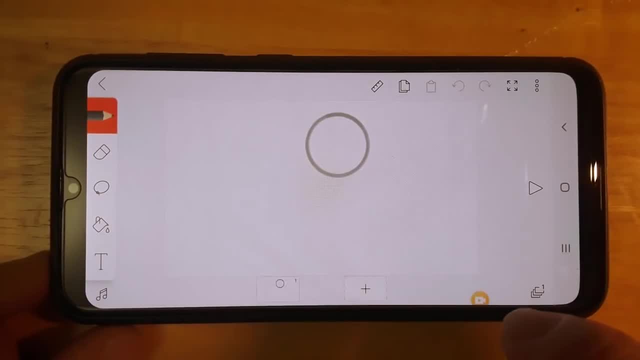 click the plus button down in your animation timeline at the bottom And this will add a new frame. You'll see a ghost of the image before. This is called onion skin and it allows us to see where we need to draw the next position in our animation To turn the 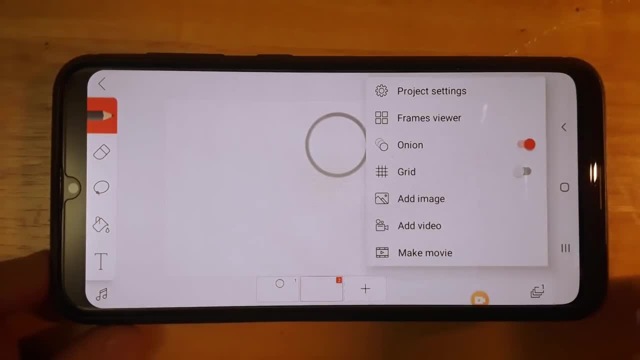 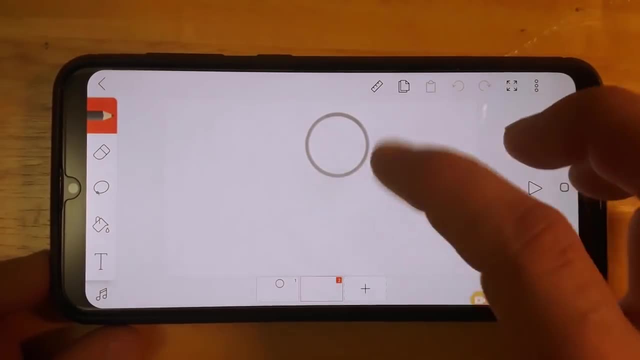 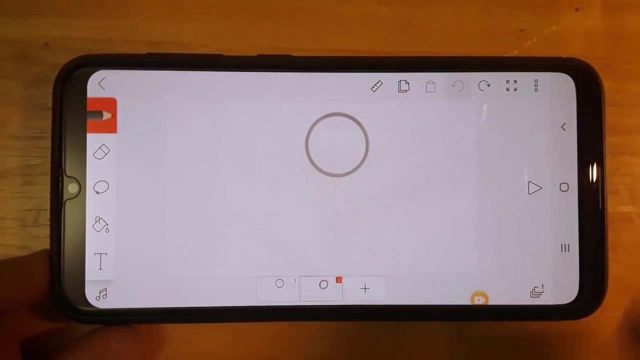 onion skin on and off. you can click the three dots on the top right and select this toggle for onion skin. And the way animation works is we're basically drawing the same thing just in a slightly different position. So for this next drawing, you can either draw the next circle or you can go back to frame. 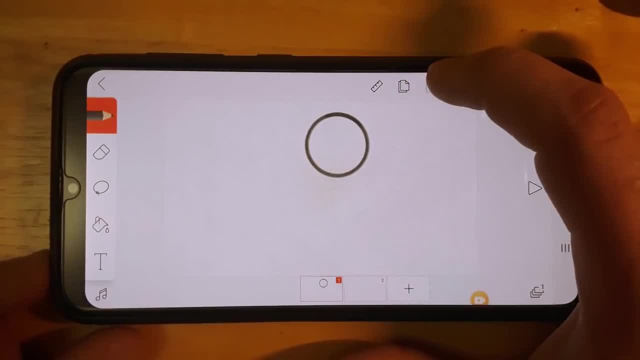 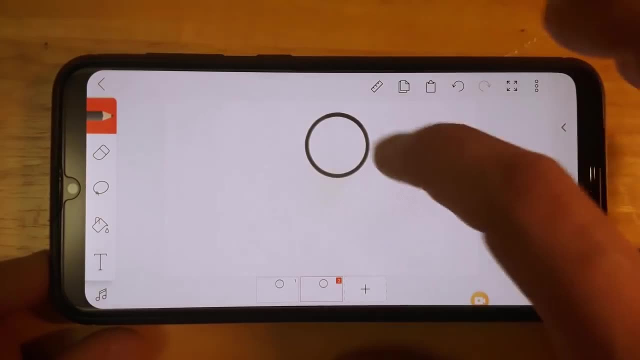 one by selecting it like so And then clicking this copy button on the top, and then go to frame two and click the paste, which is this little clipboard icon, and it'll paste the same drawing, But we'll need to move it into position, so we'll select our lasso tool. 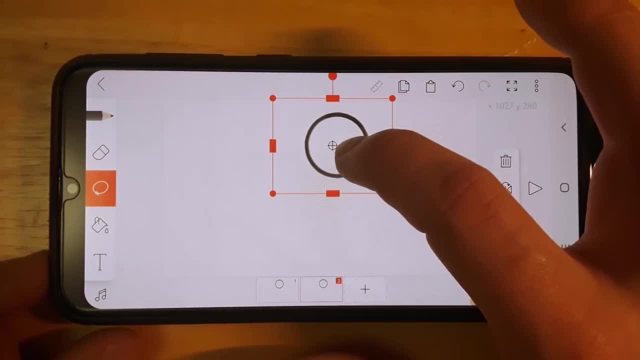 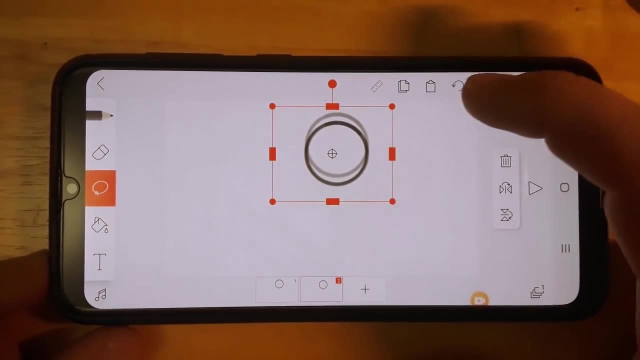 select our drawing and we'll move it just slightly down. So the way a bouncing ball works is gravity slowly affects something, right? So these first few drawings are going to be really close to each other. This is called an ease in, So we'll. 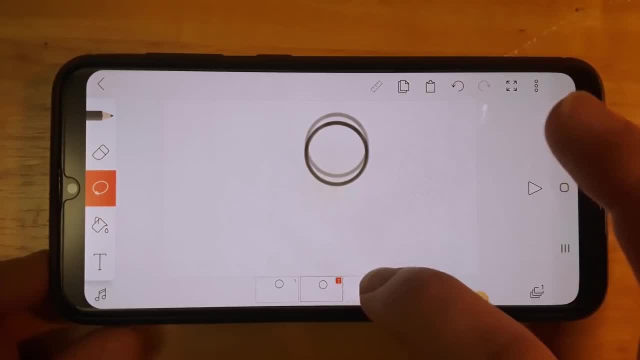 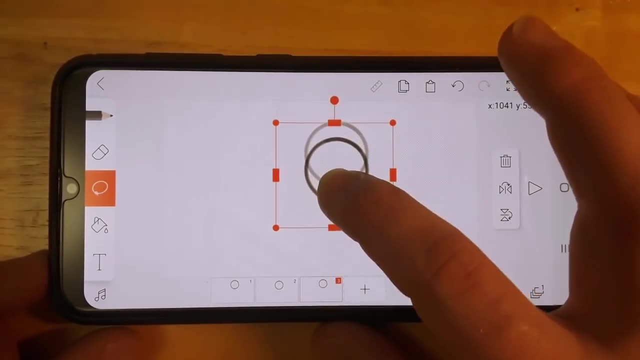 select off of it. We'll go to our next frame by clicking the plus button to add a new frame. We'll press paste again to paste that same ball, select it again, and this time we want to move it even further down. So we'll do this a couple. 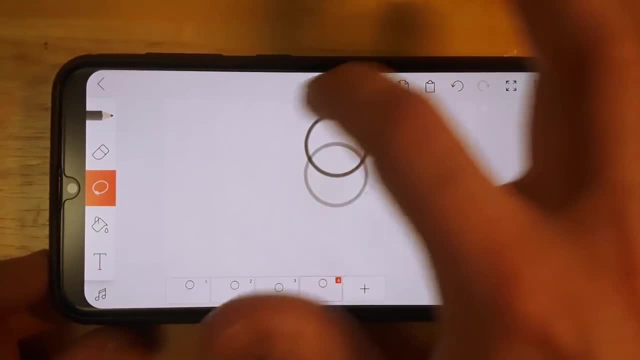 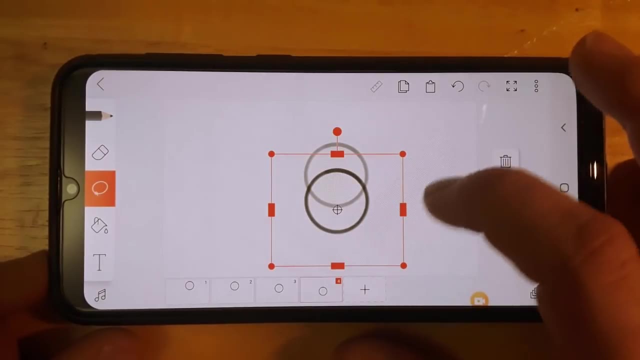 more times. I'm going to add another frame, paste it again, lasso around and then move it down, But this time we're going to do what's called a stretch drawing. To stretch this ball, we're going to squeeze it in on the sides by. 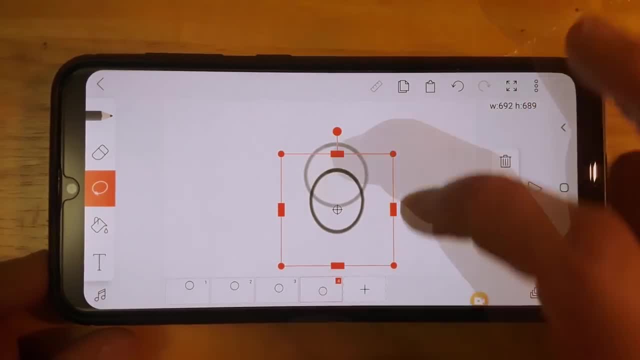 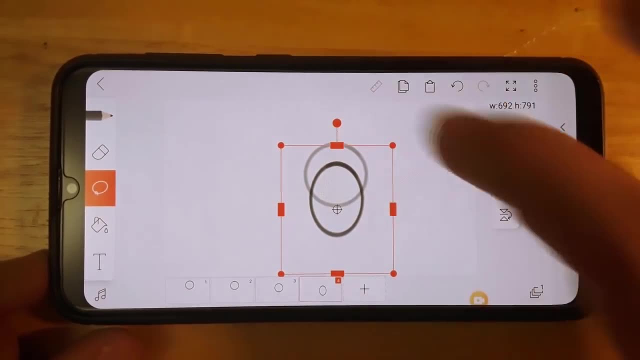 selecting the side, transform, squeezing it in a bit and then, for as much as you want to squeeze it in, you want to create an equal amount of stretch on the opposite side. So we'll stretch it out a little bit that way, and then the next drawing is going to be: 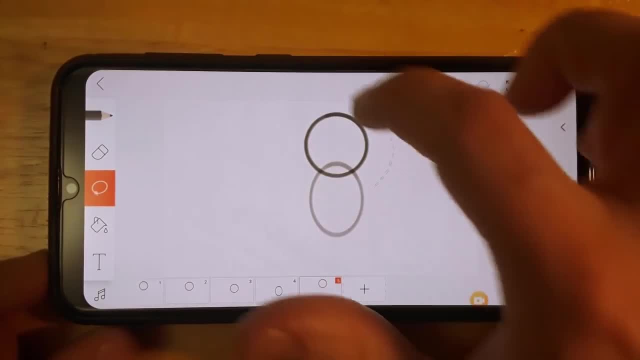 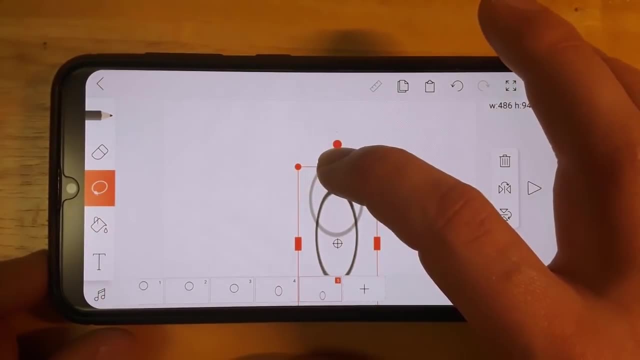 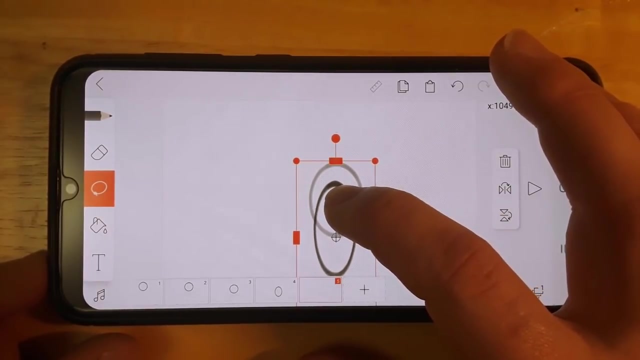 even more extreme. This will be our last stretch drawing, So squash and stretch is a very important principle in animation. Most everything moves with squash and stretch and it's a very important thing to practice and a bouncing ball is a very basic example of it. So for our last drawing, we'll have it. 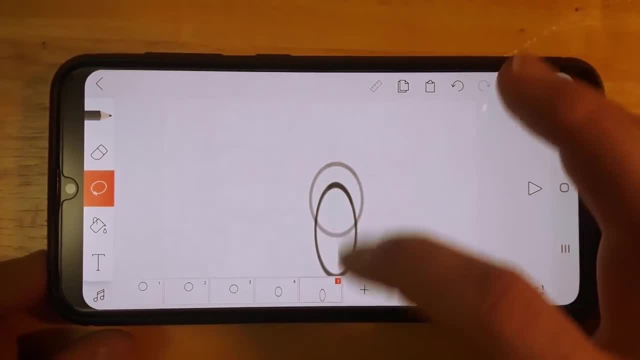 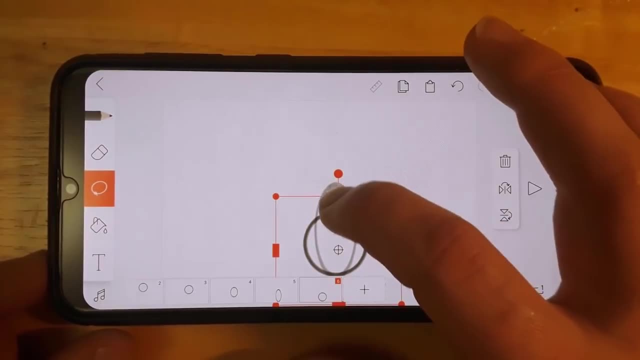 stretch all the way at the bottom, like so, And then, when it finally impacts the floor, we'll have this ball do a squash drawing. So, instead of stretching out because it's moving so fast, it's squishing down because it's impacting the ground. So we'll have it squish down, like so. So, now that the ball is squashed, 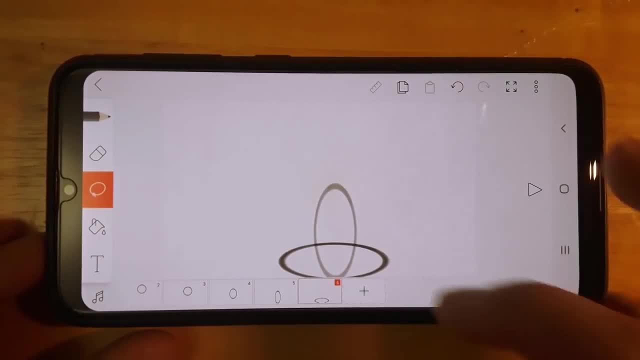 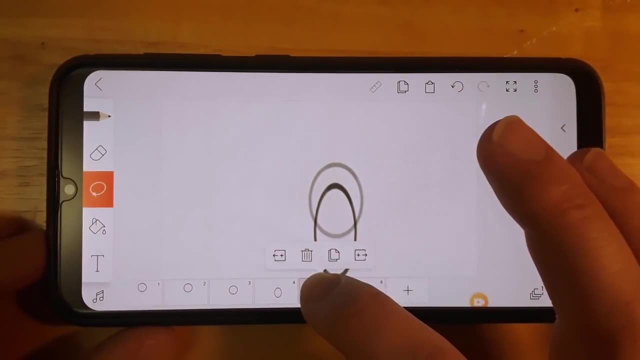 on the ground. we want to have it bounce back up in reverse order So we can draw the frames again, or we can copy and reuse the frames we've already drawn. So go back one frame, hold down your finger on that frame and you'll see a bunch of 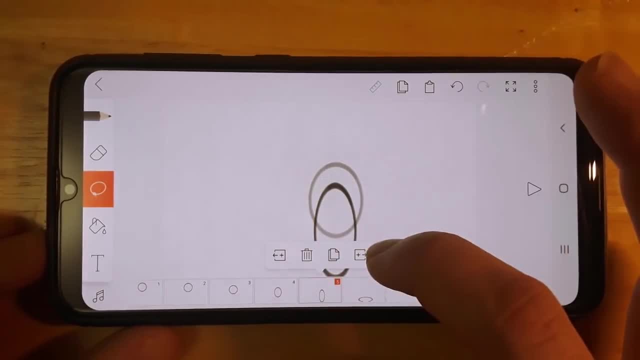 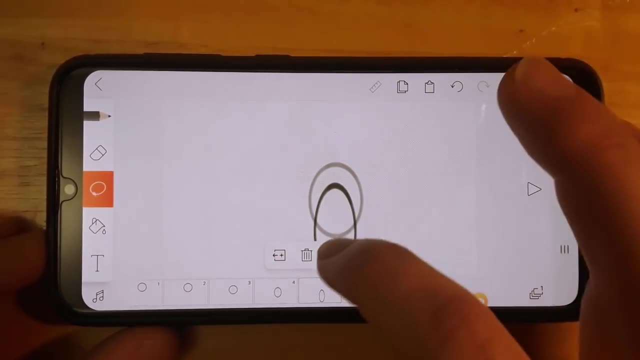 options for it. You can insert blank frames by selecting the plus buttons on the left or the right. This is good for adding in-betweens. We can delete the frame with the trash can or we can copy it with the copy button right here. So once we 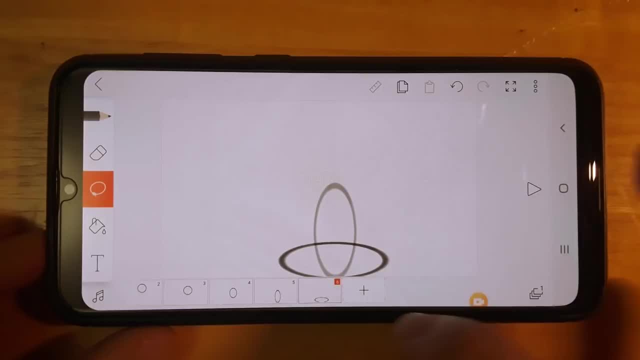 selected that we have that frame copied. Then we go back to our last frame, hold down our finger again and select the paste button with the arrow pointing to the right, And that'll paste that same drawing onto the right side. Then we want. 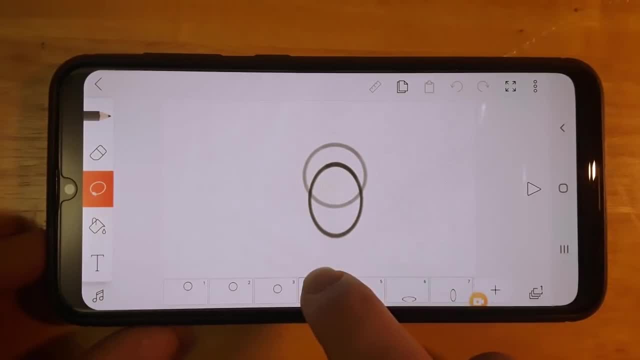 to go back one more frame, which is frame four. in this case, Hold down our finger, copy that, go to the end of our animation. hold down our finger and paste to the right And we just repeat this process until we've. 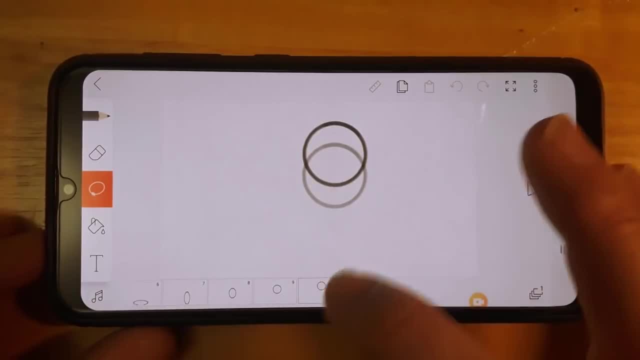 finished copying and pasting our animation to the right- And I won't copy and paste the first drawing, since that's the first drawing in our loop- To test out our animation. we can click the play button on the right here And you'll see. 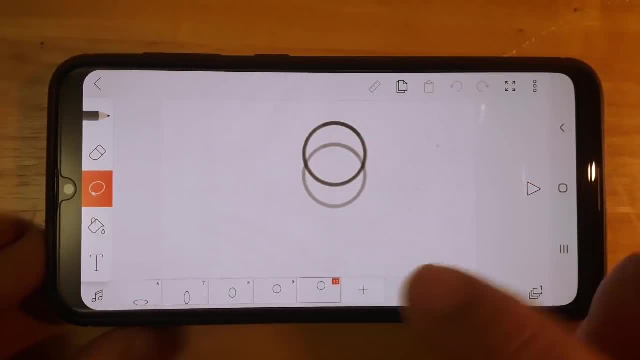 we have our bouncing ball. If we wanted to add an in-between between any of these frames to smooth it out- say, for example, from the squash drawing up to this stretch drawing, we can add a blank frame in between by holding down our mouse button and. 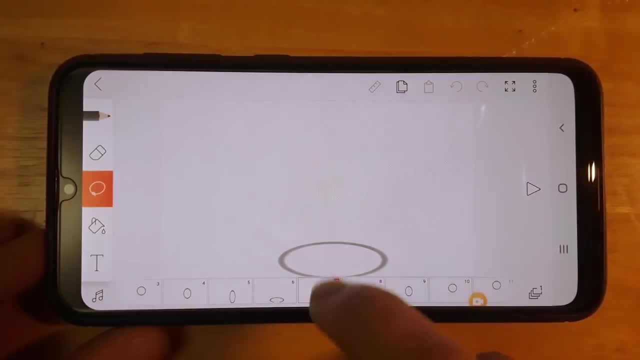 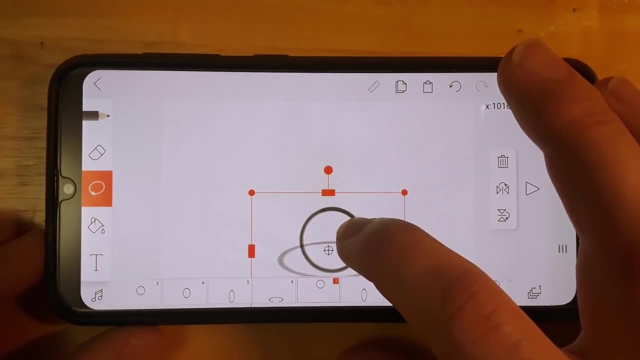 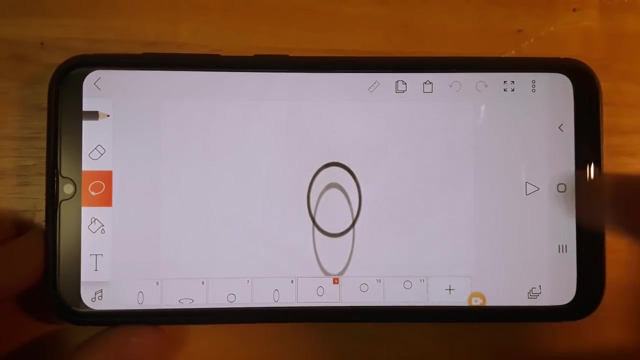 clicking the plus with the arrow pointing to the right And that'll add a blank frame in between. Then we can put an in-between by pasting our ball again and then just putting a little in-between so we can smooth it out a little bit. And now you'll see when we play our animation it's been smoothed. 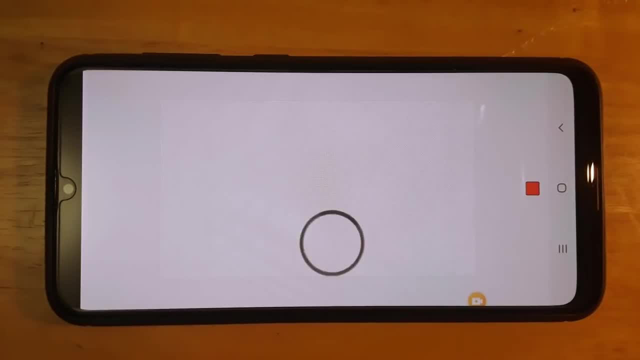 out for that frame. So that's how you can add more in-betweens to kind of smooth out your animation. Remember that the more drawings you do, the smoother your animation is going to be, but also the slower it's going to. 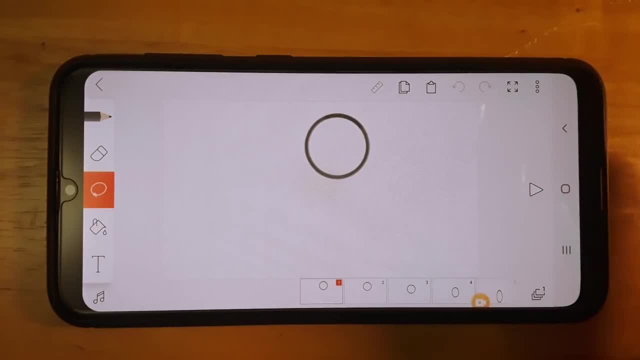 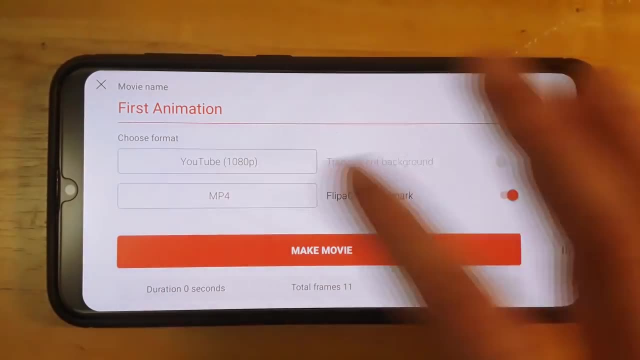 be. So now that we're finished with our animation, let's export it for YouTube. So to export your animation, click the three button up on the top right, select, make movie, and we're going to leave all these options the same, but you can change them. 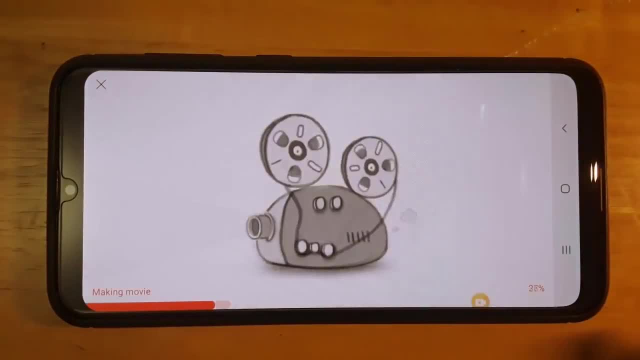 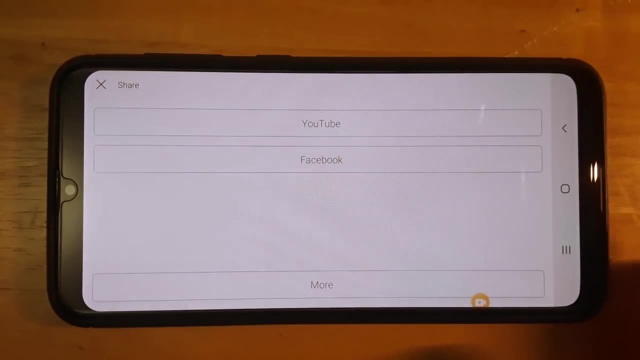 And then to start exporting it. we're going to select, make movie, And now our video has been created. If you want to upload it to YouTube, just click the share button and select YouTube from the selection here. So now that we know how. 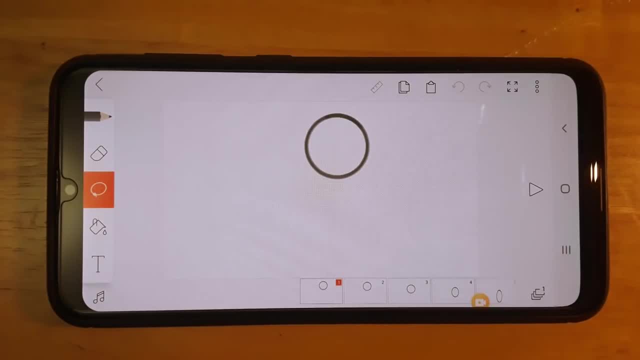 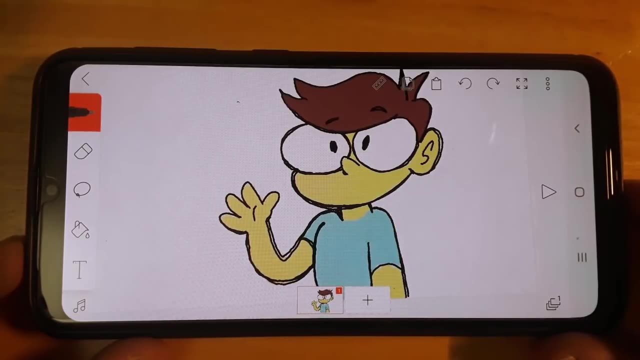 to do a very basic animation in flip a clip. let's talk about how to do a lip synced character. So we have our character already colored in, but we haven't done a mouth animation yet. To add audio to your animation, click the. 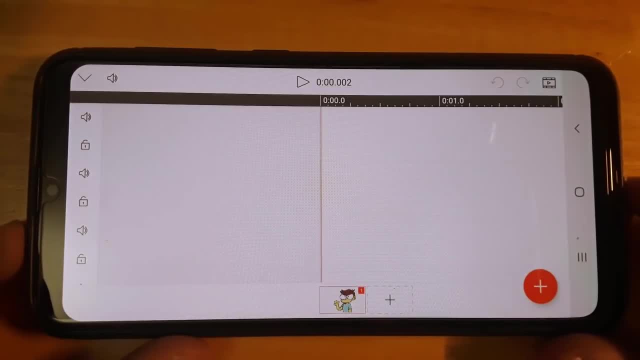 music note on the bottom left of your screen. Then to add audio, click the plus button on the bottom right and with the album picture you can add a downloaded piece of audio. or with the microphone, you can press the microphone and press. 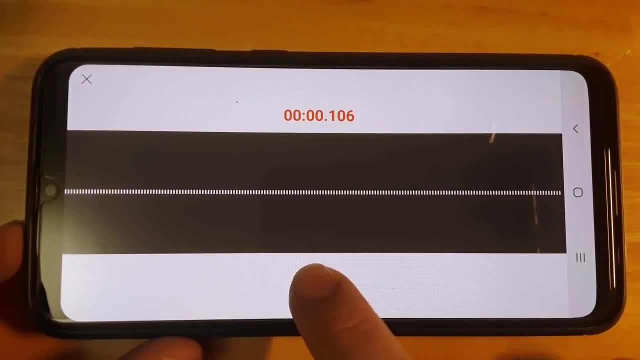 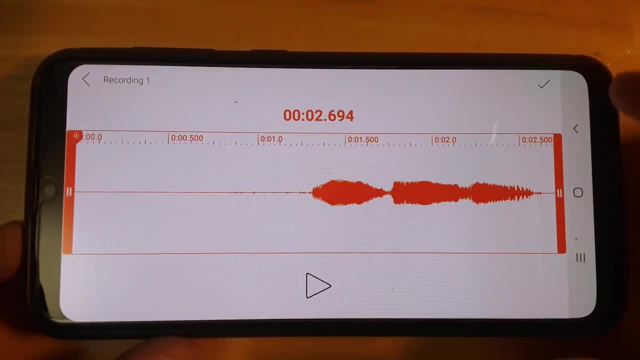 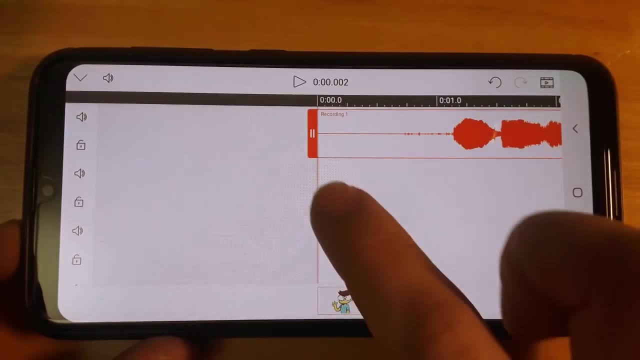 and hold to record your own audio. Let's record something right now- Why hello there? And you can play to preview your audio- Why hello there? And then press the check mark to add the audio to your animation and then drag it in to where you want it to be, And we don't need the silence at the beginning. 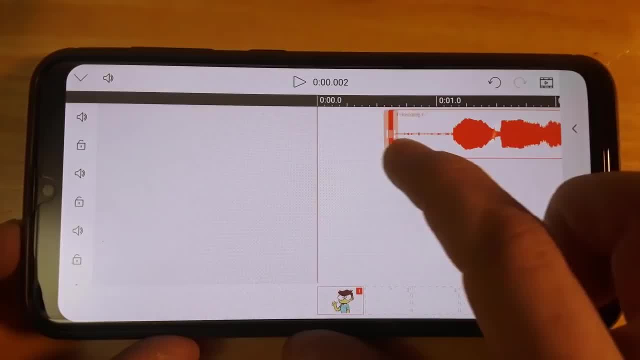 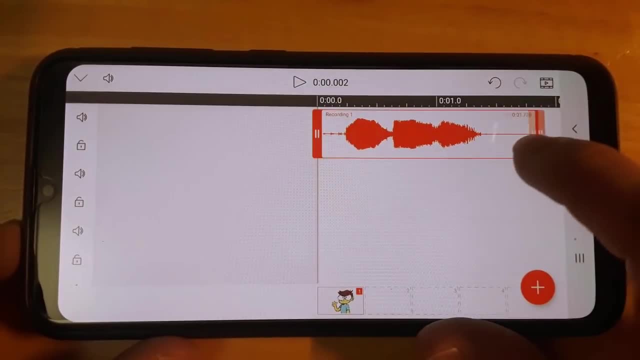 so click the audio to select it and then drag this bar to get rid of the beginning silent part And then click and drag and move your audio back to the beginning And you can also trim the silence at the end here When you're done. 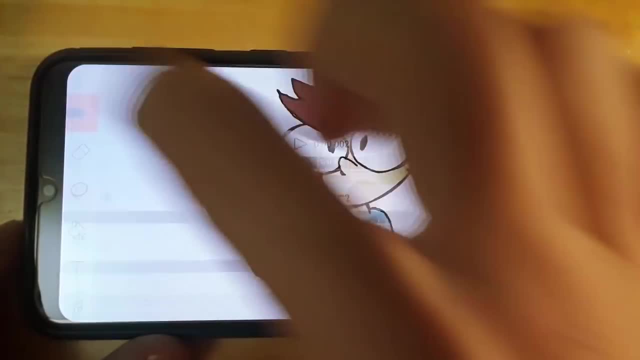 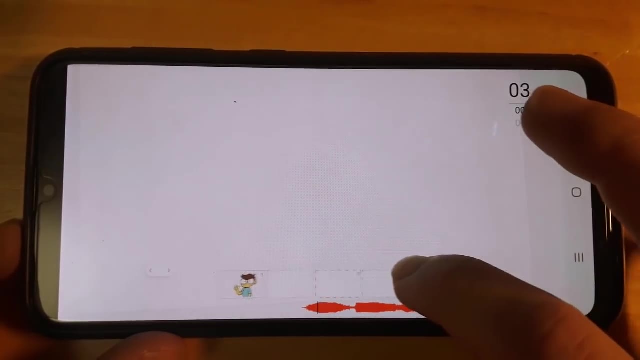 editing your audio. press the down arrow on the top left of your screen and then click the your screen and you'll see the waveform down at the bottom of your animation timeline. And if you click and drag your timeline you'll hear your audio do what's called scrubbing. 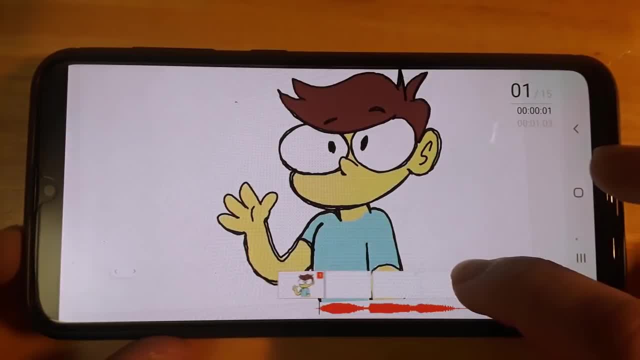 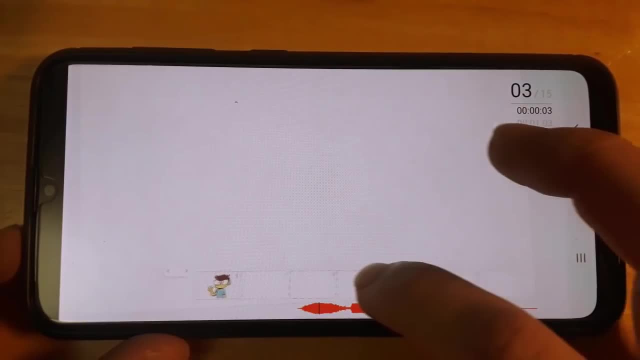 So this is how you can see what sounds you need to animate to. For example, in Y you might start with an O shape like Y and go into A and then I. So let's do that. But first off, we need to make this frame hold for as long as we want. 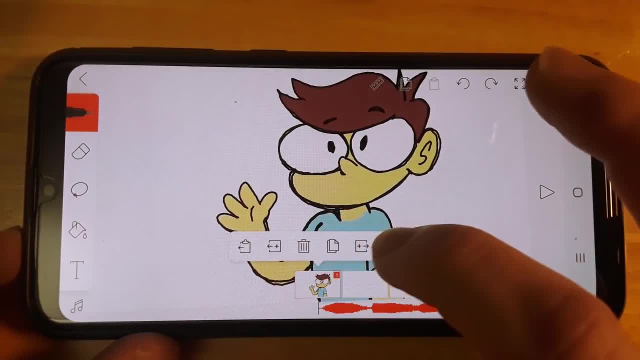 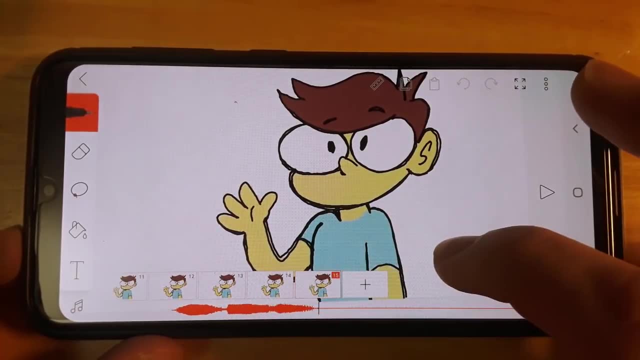 So we need to copy this frame by pressing and holding, clicking copy and then paste to the right And keep doing that until you've covered your entire animation. This is how you create a hold frame. If you wanted your character moving, you would want to animate your moving character before. 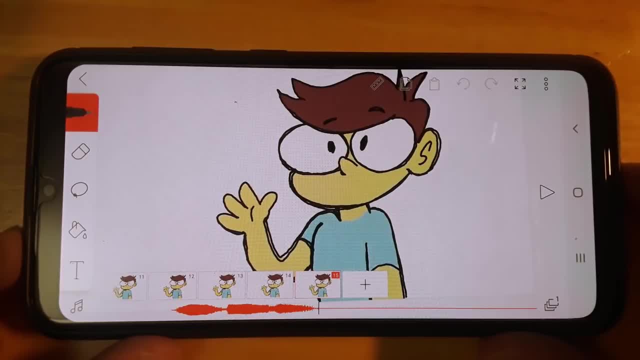 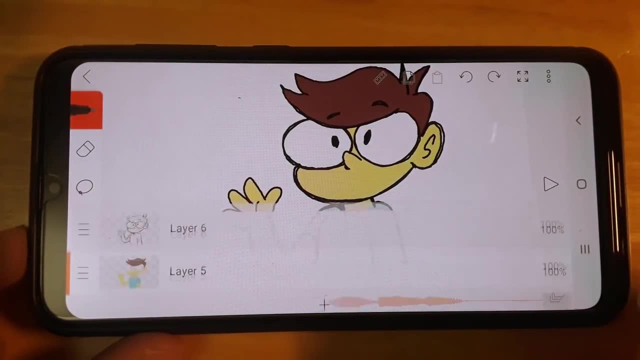 doing any lip sync. Lip sync is really something you should do at the very end of your animation. So now that we have our hold frame all created, let's create a new layer. So click our layers button, press the plus to create a new layer and we'll call this: 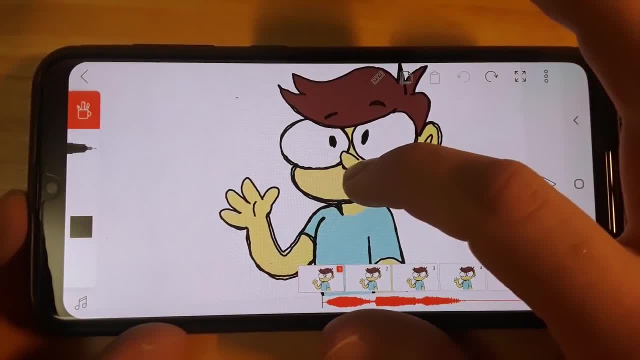 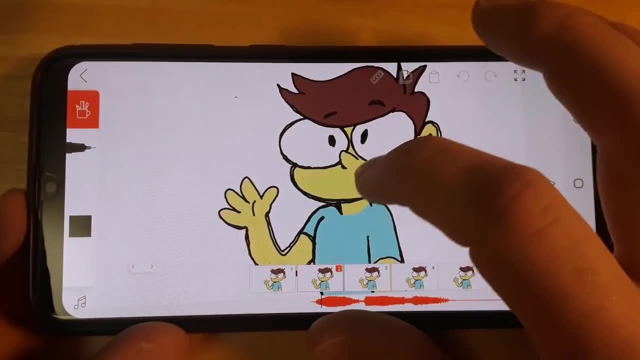 layer mouse And for the first frame we'll do a closed mouth shape with just a smile And then we'll scrub through our audio to see what frame number two sounds like. So we're going to make an O shape and we can zoom in to better draw our mouth, so we can.